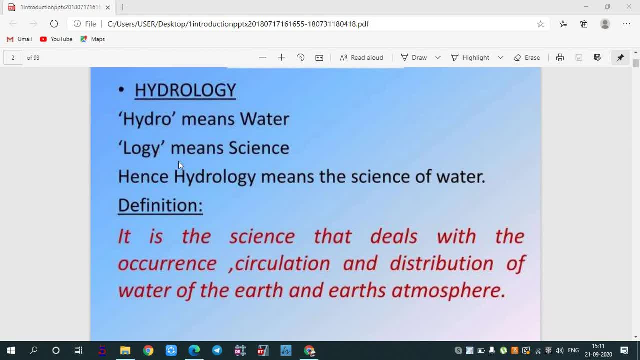 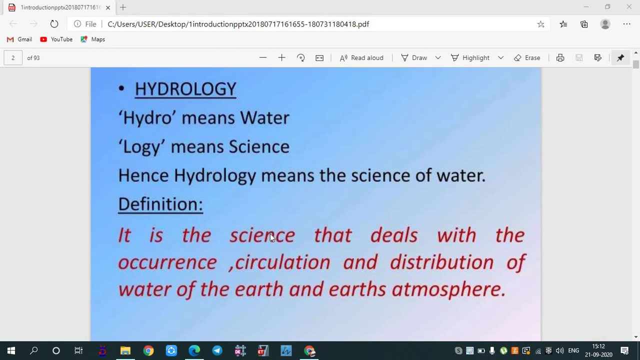 Good morning everyone. So we are starting today with the new subject, that is, hydrology. So this is also related with water Basically, as you all know that hydro basically means water and logi means science, So together it becomes hydrology. Okay, So basically it is a science related to water. So by definition it can be said that it is a science that deals with the occurrence, circulation and distribution of the water of the earth and the earth atmosphere. So it is clearly mentioned over here that it basically deals with what: the occurrence, the circulation and the distribution of water on the earth and in the earth atmosphere. 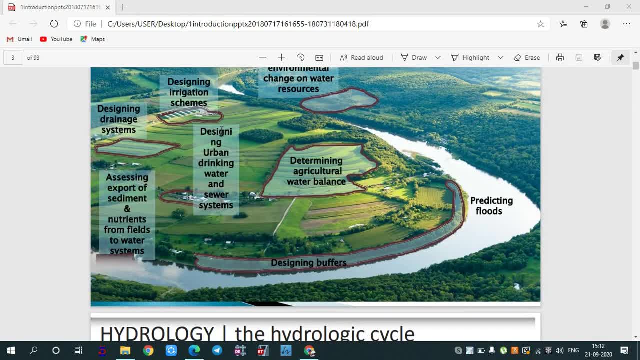 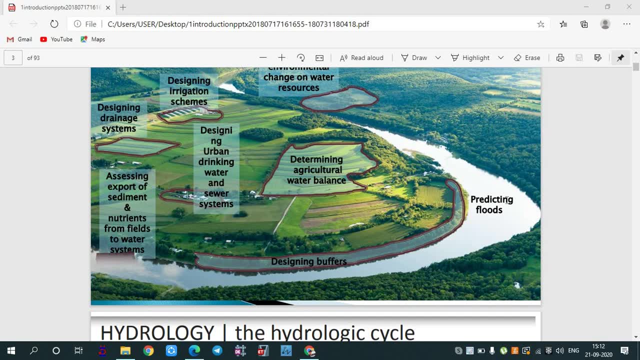 Okay, Hydrology. There are various applications of hydrology, since it has been used, Related to water, So it can be used in prediction of floods. It can be used in designing of buffers- Buffers are basically nothing but the area which has been on the sides of the streams, that are nothing but your buffer. For agricultural water balance. it can be used, since it is related to water, For designing urban drinking water and sewer system. Okay, Now assessing export of the sediments and nutrients from the water system. Okay. 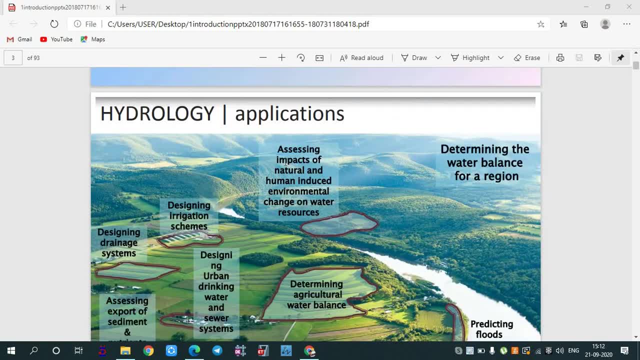 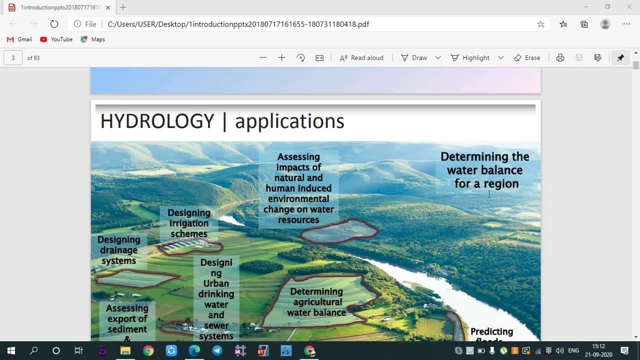 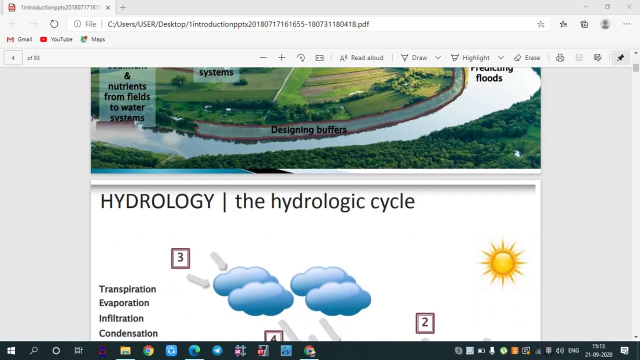 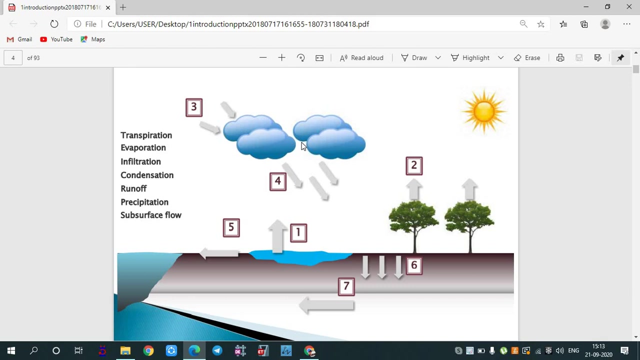 Designing drainage system. Designing irrigation scheme: Okay. Assessing impact of natural and human included environment changes on the resources and determination of water balance for it. So these are the various applications of hydrology. Okay, After that, this is a hydrological cycle which you have studied in your schools also, Okay. 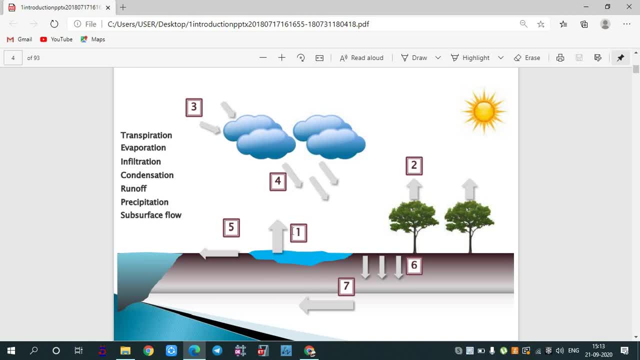 First step is nothing but evaporation, As you know that most of the earth is covered with water. So, because of the temperature, because of the high temperature, Because of, during the summer season, what happens? The water from the streams, lakes, oceans get evaporated. 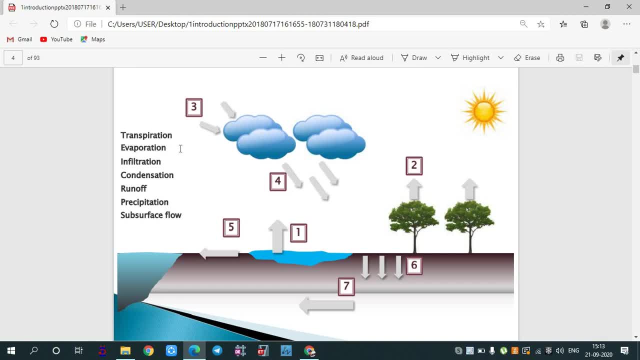 Okay, After that, the second step is evapotranspiration. Okay, That is. first is your evaporation, Second is your transpiration. you, as you know that your plants and your trees also require water. some water flows in the leaves and some parts of the roots, so they that water also get evaporated. that is nothing but your. 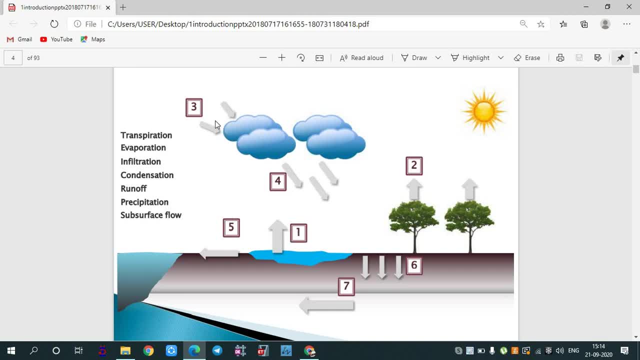 transpiration. okay, after that, the third step is your condensation. after that, these water in the evaporated form condense and form a cloud. okay, after that, what happens? third process is your condensation. after that, this condense cloud, what happened? a create rainfall. okay, that is in the 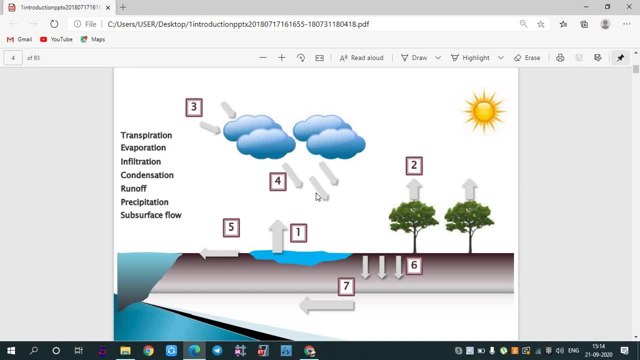 form of what? precipitation? fourth step is your precipitation, okay. fifth step is what some water gets collected into the stream. some water flows. that is your runoff, okay. now six step is your infiltration. some water get what it gets inside your ground. that is your runoff, your infiltration, okay. some water flows inside the ground, that is your subsurface flow. so this, 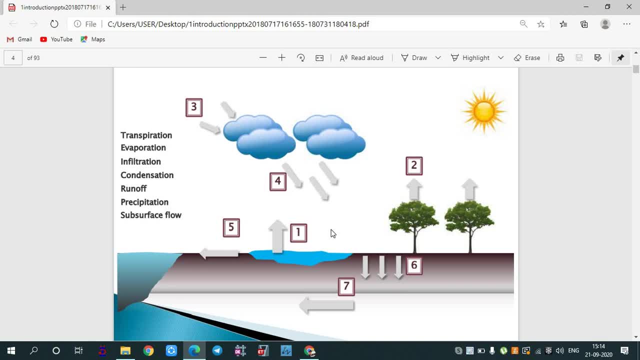 is basically your hydrological cycle. okay, the first step is evaporation. second step is your transpiration. transpiration, basically, is nothing but whatever the water gets evaporated- from trees, leaves- that comes under transpiration. after that, whatever the water gets evaporated, that form a condense after condensation reforms rainfall, and it is in the form of precipitation. 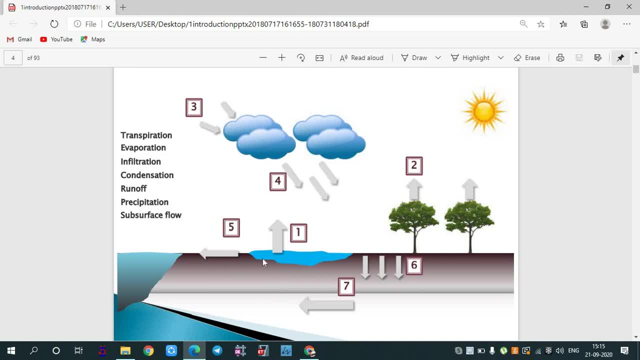 after that, some water gets converted into runoff, okay, some water gets infiltrated, that is, inside the ground, and some water flow below the ground, that is your subsurface. so, basically, this is the hydrological cycle. okay, so this is the process: evaporation of water from the surface source. like river evaporation happens from. 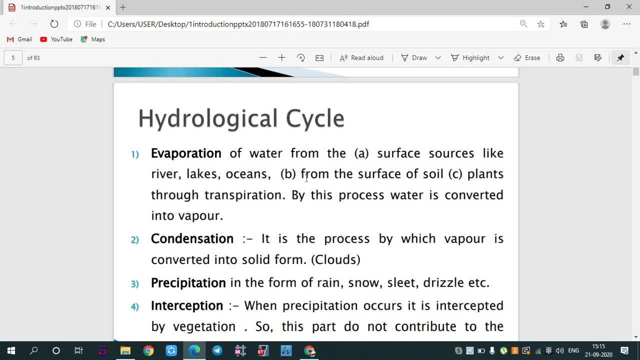 where sources like river lakes, oceans, okay, from the surface of the soil, plants, through transpiration, as i've told you, from plants, the water which gets evaporated is nothing but your transpiration. by this process, the water is converted into vapor. after evaporation and transpiration, it gets 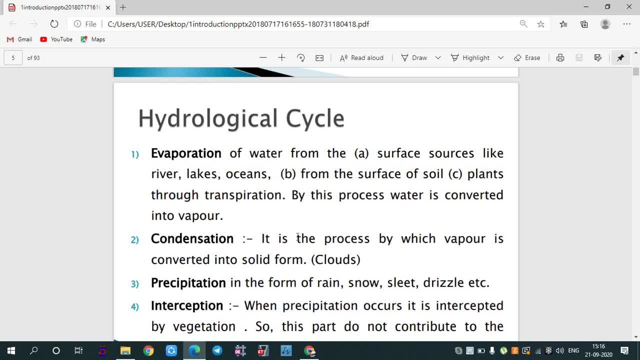 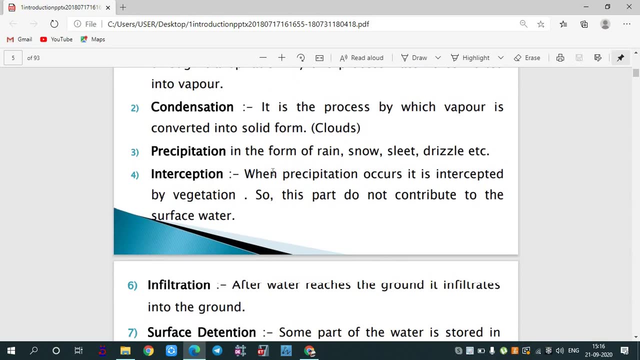 condensation. it is in the process by which vapor is converted into solid form, which forms clouds. okay, then precipitation. after the condensation, precipitation happen in the form of rainfall, snow, lead drizzle, etc. okay, after that precipitation, some part of the water gets. what get? insights? interception is also one of the part. it is not mentioned in the 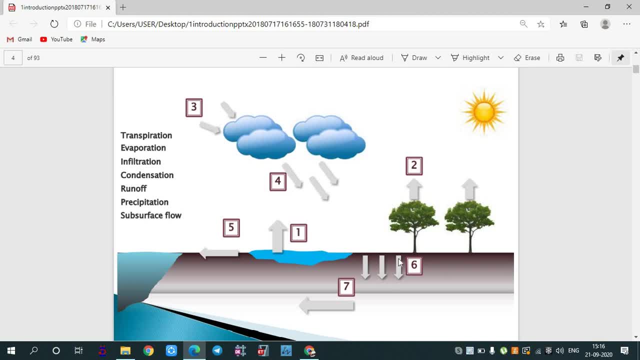 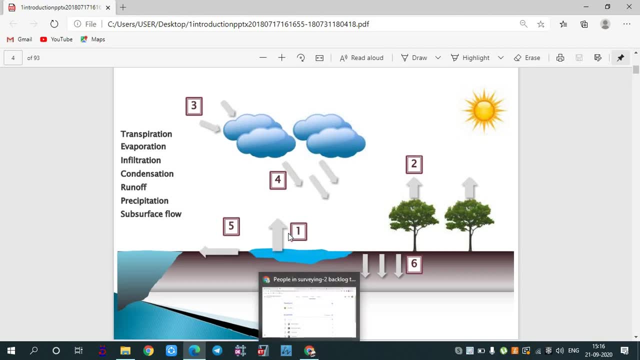 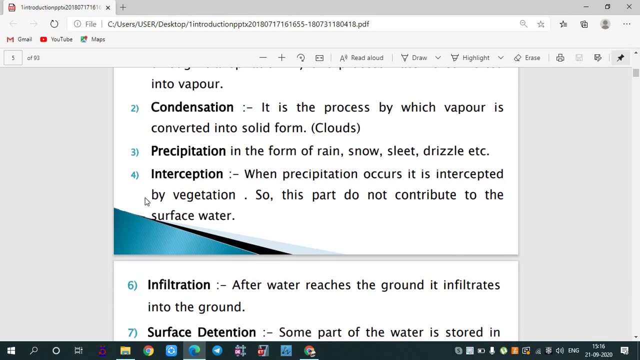 cycle interception. basically the whole water does not go inside the ground. some water stays on the leaves or some parts of the plants, okay, so basically that part is nothing but your interception. when the, when the precipitation occurs, it is intercepted by vegetation. so, as i have told you, some plants, what happens? some water gets inside that plants. also, that part is called your. 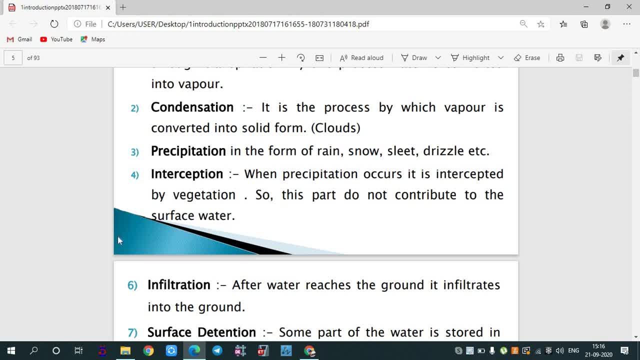 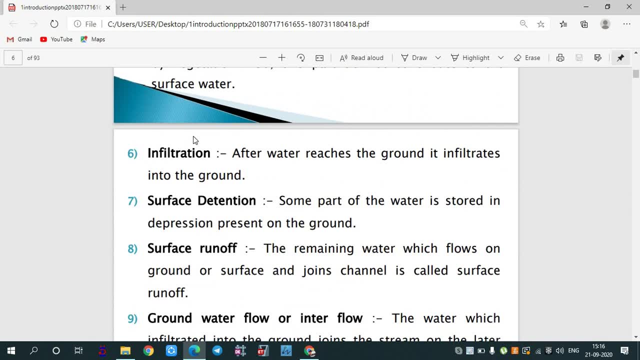 interception, so the part do not contributes to the surface water. okay, so that part is taken into another term and it has been provided into given another term that is called interception. okay, after that infiltration, some water gets what infiltrates into the ground. that is your infiltration. okay, after that there is surface retention: some part of the water is stored. 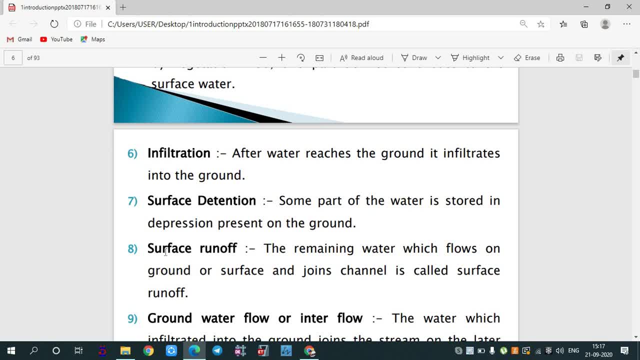 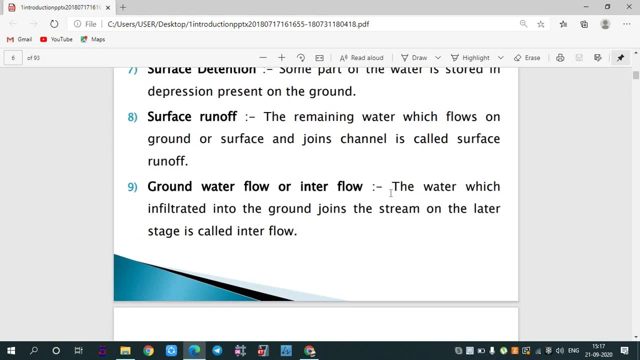 as you know, that groundwater table, some water gets stored inside the ground. okay, then there is surface runoff. the water in excess gets flows on the ground. the remaining water, which flows on the ground or the surface and joins the channels, is called as what runoff. after that, groundwater flow, or interflow the water which infiltrates. 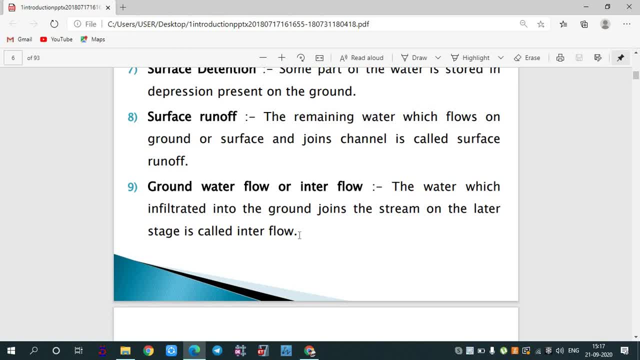 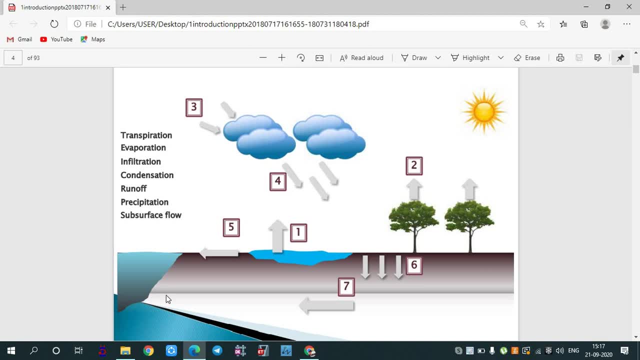 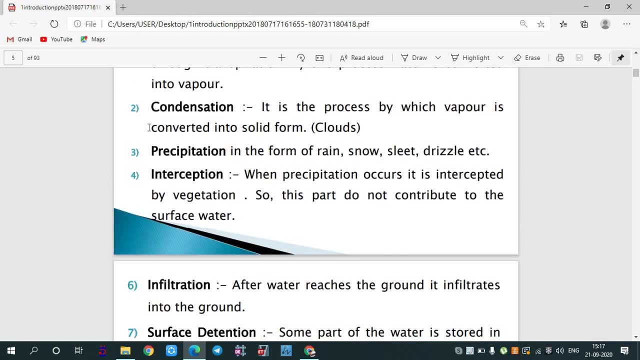 into the ground, joins the stream, on the later stages called as interflow. basically that is your subsurface flow, some water from the ground also what contributes towards the channel, that is your interception, interflow or you can say groundwater flow. so this was the eighth or total nine step of your 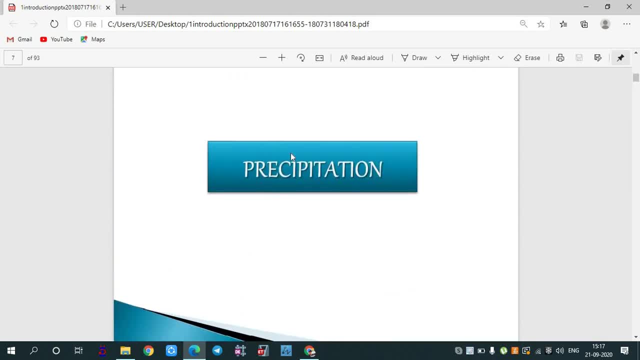 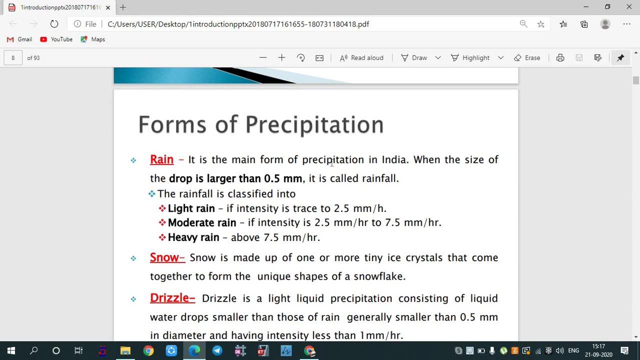 hydrological cycle. after that we will study about precipitation in detail. so precipitation, as you know, the main form of precipitation is your rain. it is one of the main form of precipitation in india, because we are starting, related to indian hydrological cycle. so basically, in india, the main 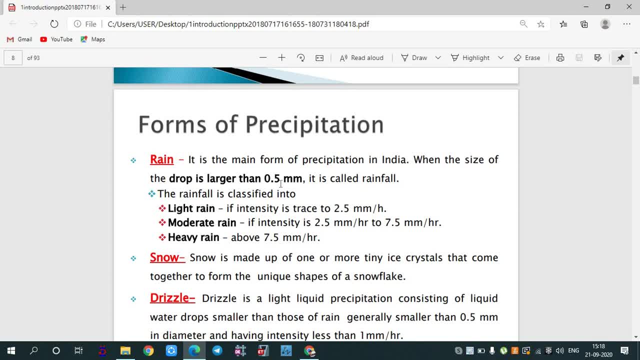 form of precipitation is rainfall. when the size is larger than 0.5 mm, it is called as rainfall. it is when the drop of the rainfall is more than 0.5 mm, then it is called as rainfall. if it is uh less than this, it would be considered into some different category. 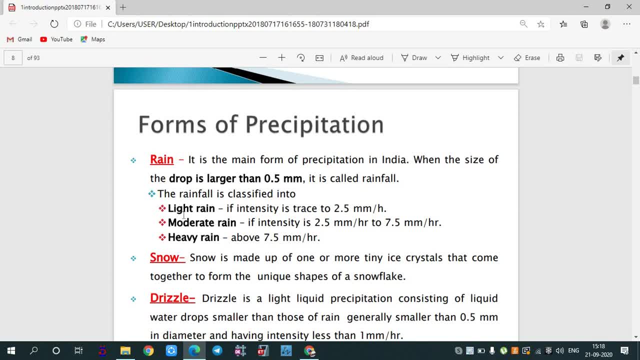 here we have been given the classification regarding the rainfall: which rainfall is considered as light, moderate or heavy rainfall. so if the intensity trace is 2.5 mm per hour, then it is called as light rainfall. so if the intensity is less than 2.5 mm per hour, then it is called. 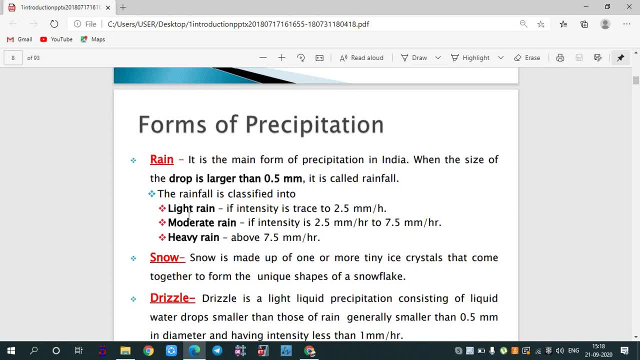 which rains 2.5 mm per hour, then it is called as light rainfall. If it is between 2.5 mm per hour to 7.5 mm per hour, then it is your moderate rain, and above 7.5 mm per hour it. 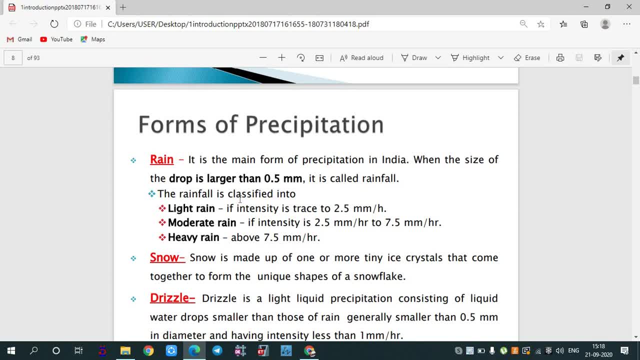 is considered to be heavy rain. So this is the classification of rain. After that, another form of precipitation, as you know, it is in the form of snow. Snow is made up of one or more tiny ice crystal that comes together to form a unique shape of snow. So, basically, 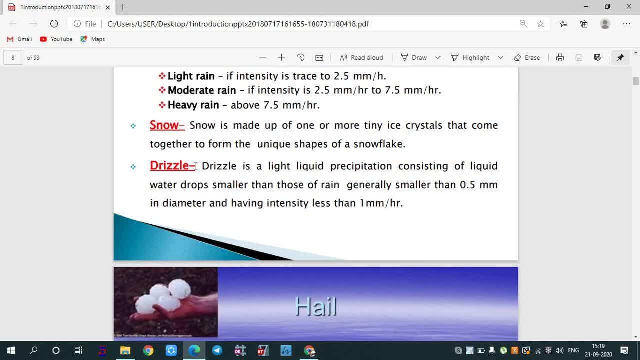 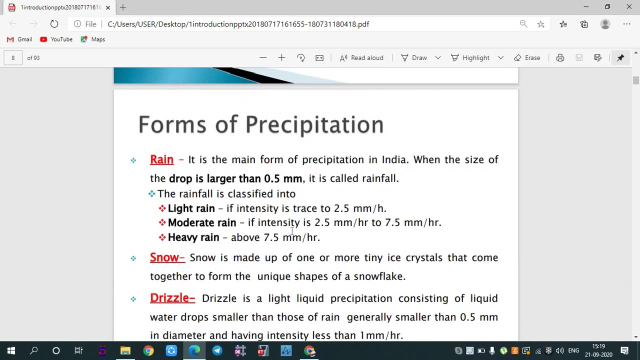 it is nothing but your ice crystals. Then another form of precipitation is drizzle. Drizzle is a light liquid precipitation consisting of liquid water drops smaller than those of the rains, generally smaller than 0.5 mm. So, as I have told you, above 0.5 mm it is considered. 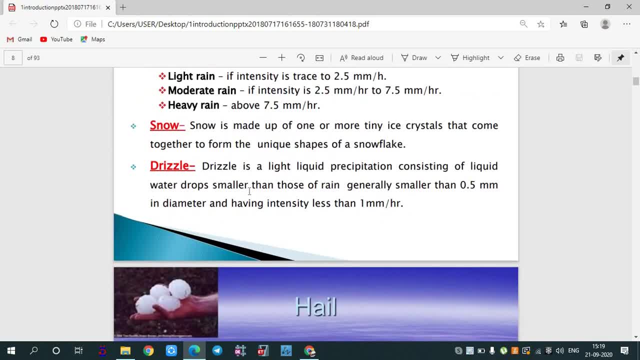 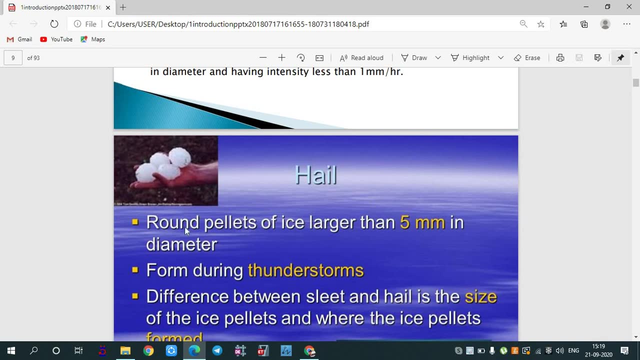 to be rain below 0.5 mm, it is considered to be drizzle In the diameter. I am having intensity of less than. So drizzle basically has an intensity less than 1 mm per hour, Then another form of precipitation is your hail. You must have seen this round petal of ice larger than 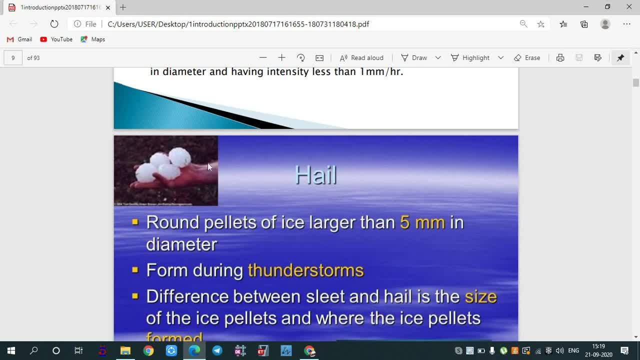 5 mm is in diameter. Sometimes, precipitation also happens in the form of round petal ice, which is generally 5 mm, which is having a size of 5 mm in diameter. This generally happens during thunderstorm. The difference between thunderstorm and thunderstorm is that the temperature of thunderstorm is. 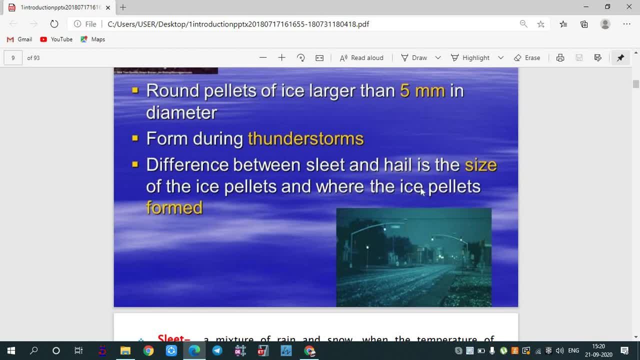 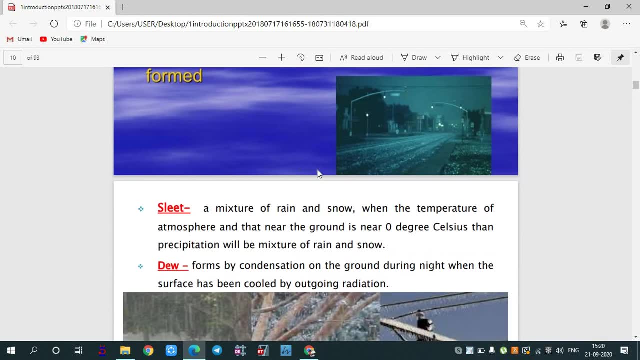 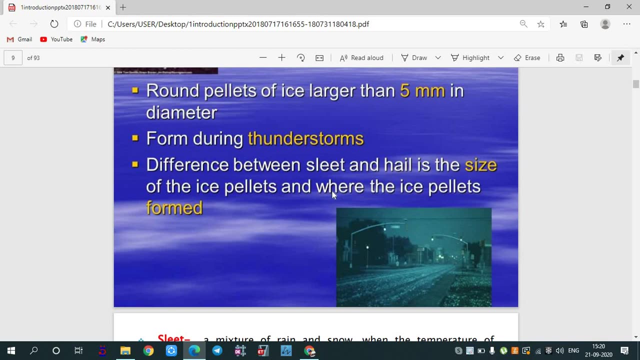 between sleet and hail is the size of the ice petal and the ice petal form. So if it is larger than 5 mm, then it is called as what hail And then sleet, a mixture of rain and snow. If the size, if it is raining as well as and there is a form of some quantity of. 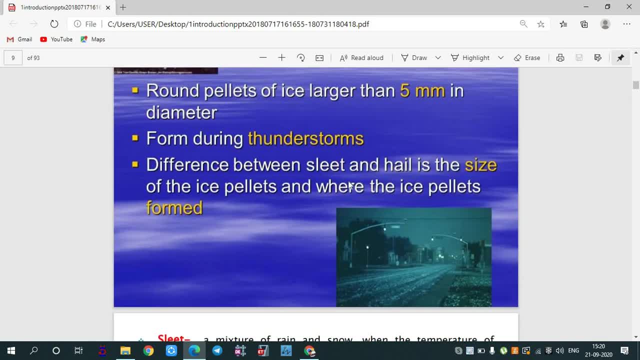 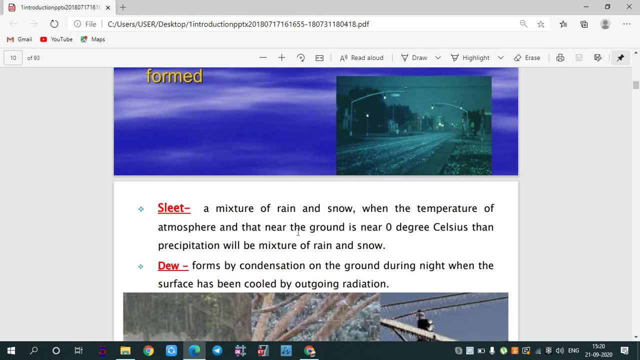 hail is there, So, and if it is having a size less than 5 mm, then it is considered to be a sleet. It is a mixture, basically, of snow and rain, So when the temperature of the atmosphere and the near the ground is near is 0 degree. 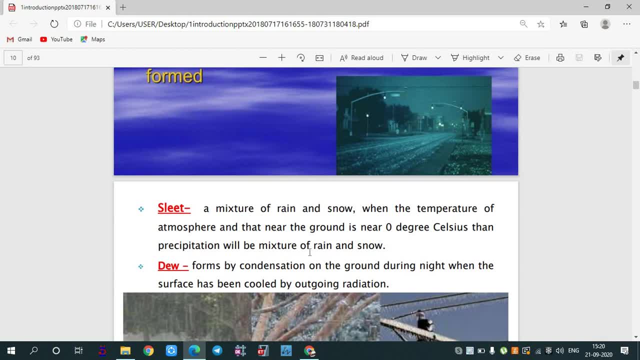 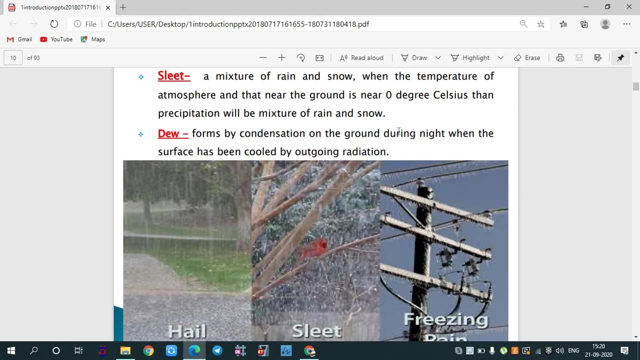 Celsius, then the precipitation will be in the form of mixture of rain and snow. So, basically, this happens when your ground temperature is 0 degree Celsius. okay, The next part of your precipitation is the deal formed by condensation of ground during the night, when the surface 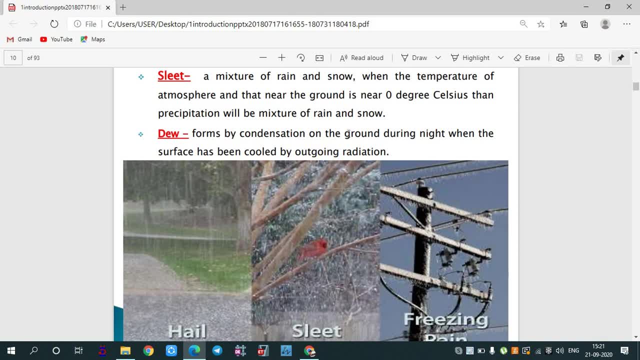 has been cold by outgoing radiation. So basically, this happens on the ground. You must have seen early morning. you find some dew on your seats of your vehicles or on your plants. you can see that there is some form of water is over there. this is because of condensation of of the ground during. 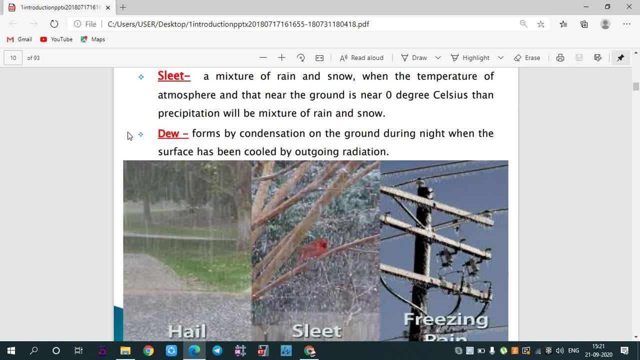 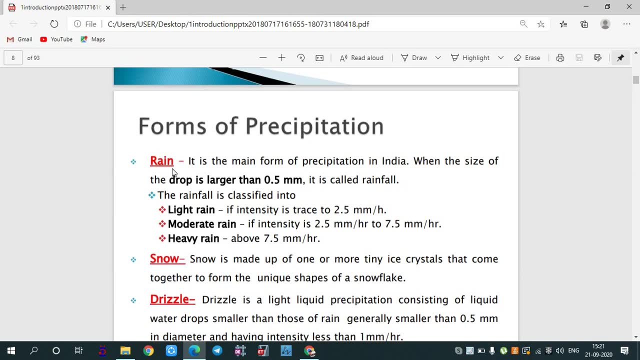 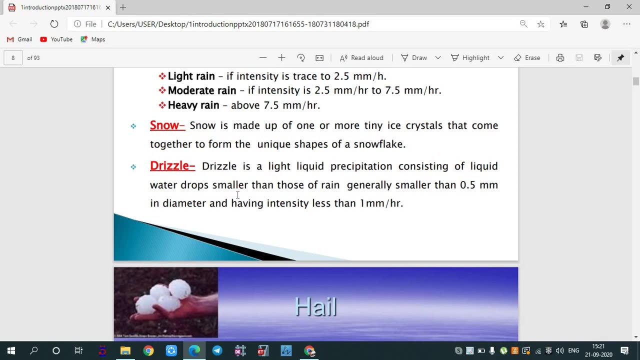 the night time, because the temperature during the night time get decreases, so there is a formation of dew. so these are the form of precipitation. rain is the form of precipitation. this is the main form of precipitation. snow is another form. drizzle, I have told you, if it is less than 0.5 mm. 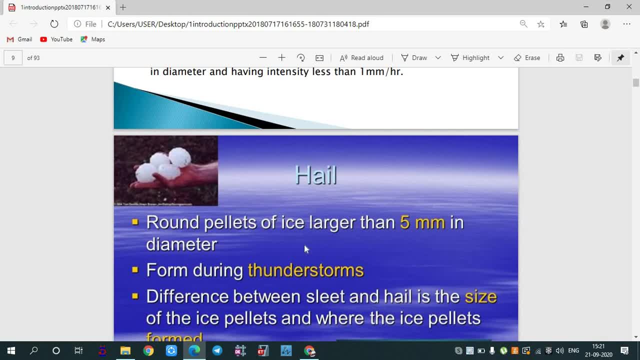 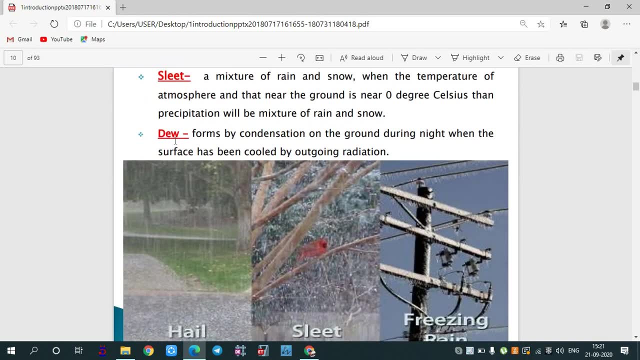 then it is considered to be drizzle, then it is hail which is 5 mm in size. if it is less than 5 mm and it is in the form of rain and snow, then it is considered to be sleet. and the last one is your. 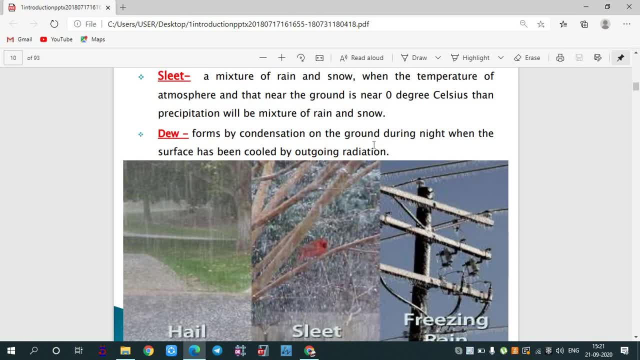 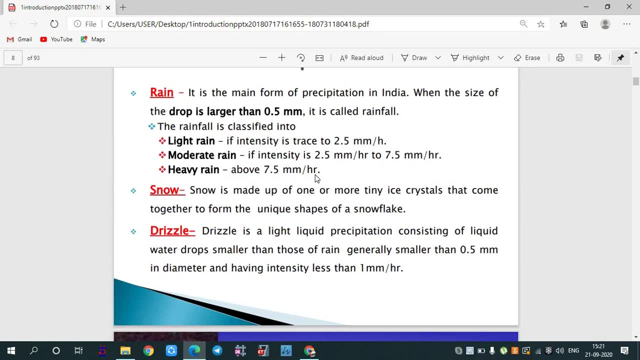 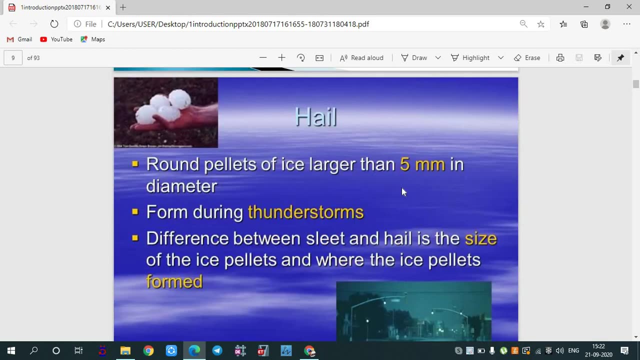 dew, which is generally happened on the ground because of the less temperature during the night time. okay, so these are the all different forms of precipitation. as you can see over here, there are different diagrams given over here. you can see, over here it is just ice crystals which is only having a size of 5 mm, then there 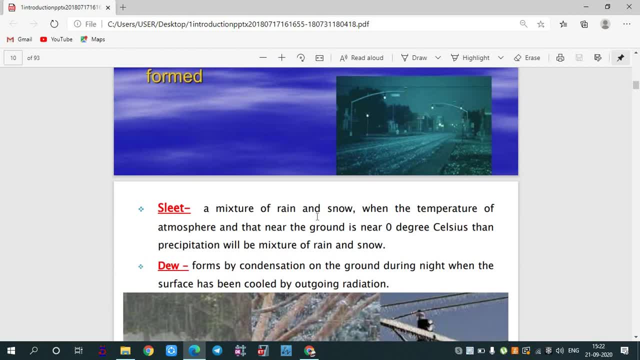 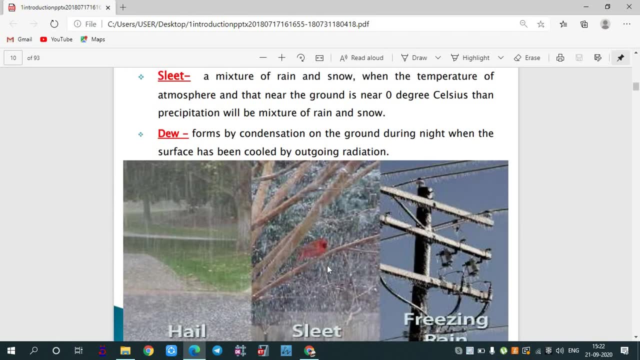 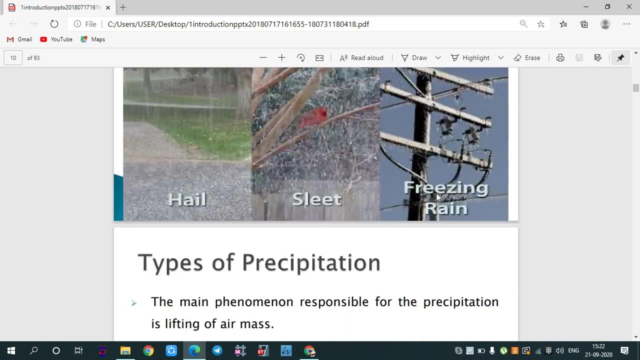 this is. this is another photograph of your hail and this is another form of your hail, and here you can see that there is a forming of sleet, there is some snowflakes which is having size less than 5 mm, and as well as there is raining also. okay, so this is another part: freezing rain. 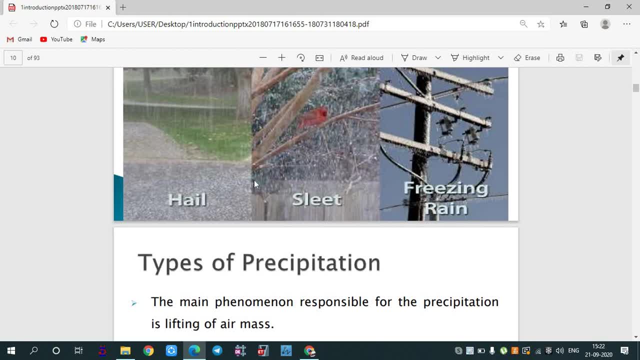 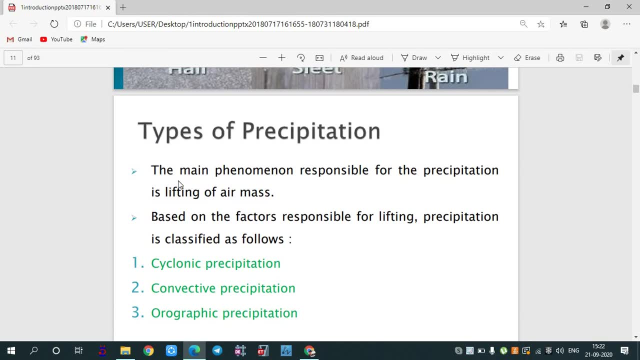 so this is all about your precipitation, or in the forms of precipitation. now we will discuss about the types of precipitation. okay, the main phenomena responsible for precipitation is lifting of the air mass. as you all know, the air mass get lifted up over there, they get condensed, they form cloud. 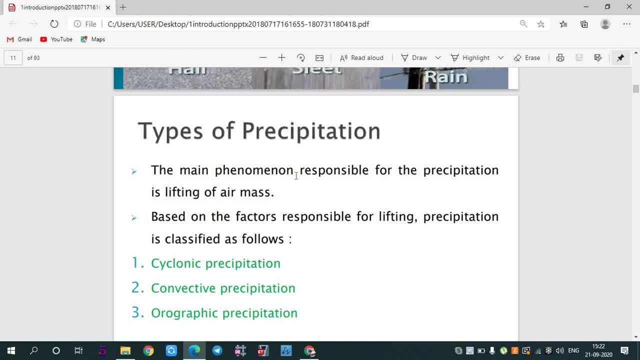 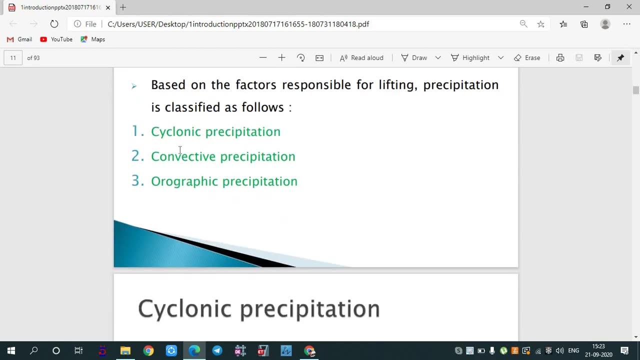 and after that your precipitation happens. okay, so the main phenomena responsible is what precipitation happen because of lifting of air masses. okay, so, based on the factor responsible for lifting, the factor which are responsible for lifting, the precipitation is classified as follows: a. there are three category. one is your, cyclonic precipitation, one is your. 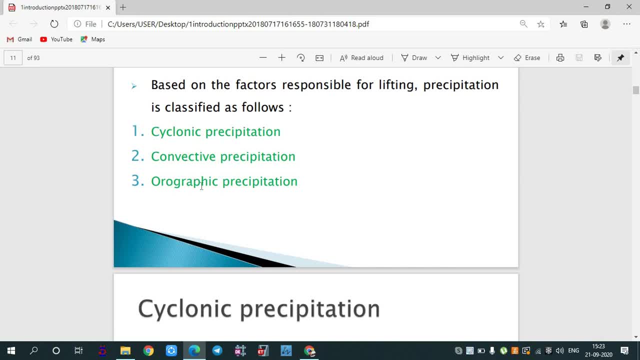 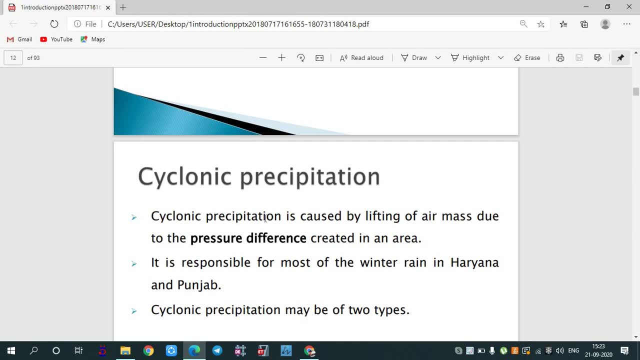 convective precipitation. third, is your orographic precipitation? okay, we will discuss each of them in brief. cyclic precipitation: this why it happen? because cyclonic precipitation is caused by lifting of airmass due to the sleeping為yl, 우산 머 turnover due to. 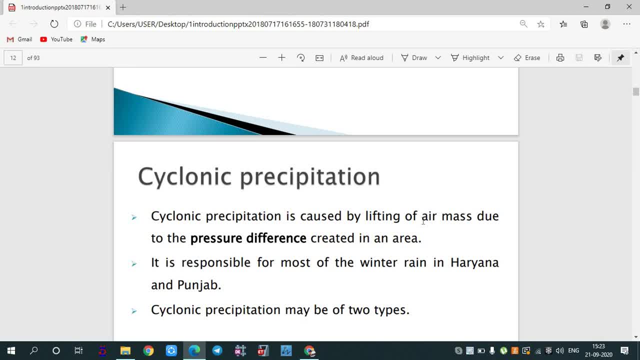 the pressure difference created in the area. so this capacity happens because the air mass get lifted up with those of the pressure differences that cause bymoulning the air mass. so when it is created this will distribute the earth of the air mass as the air crispy will churn. 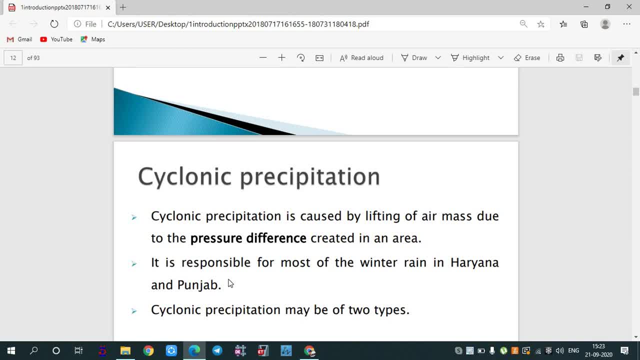 and then it will cannot chocolate perfect, and that is possible because, due to thejähral created in the area- okay, this mainly happen- it is responsible for most of the winter rain in haryana and punjab. so this is the main reason in uh, this is the main reason why in during winter, 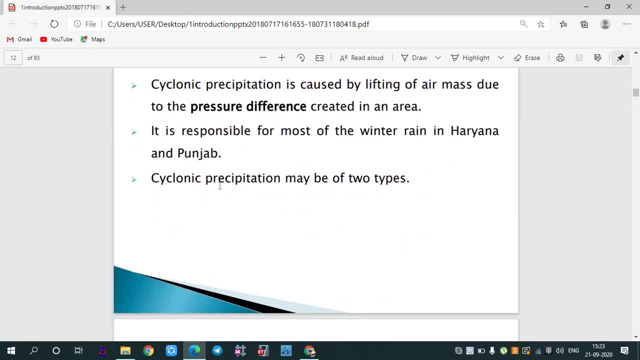 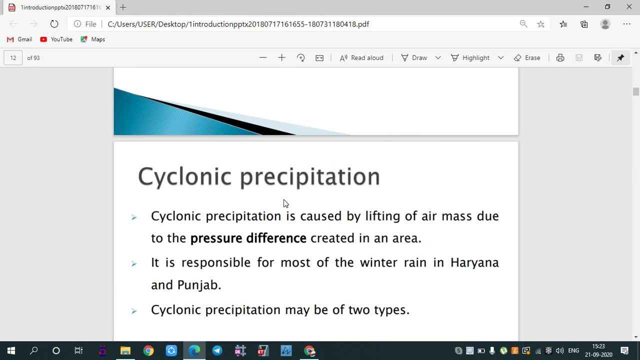 uh rain is generally happening in haryana and punjab. uh cyclonic precipitation can be categorized into two category. okay, so the basic phenomena is that the air mass get lifted because of the pressure difference. that you must know. it happens because of the pressure difference created in the 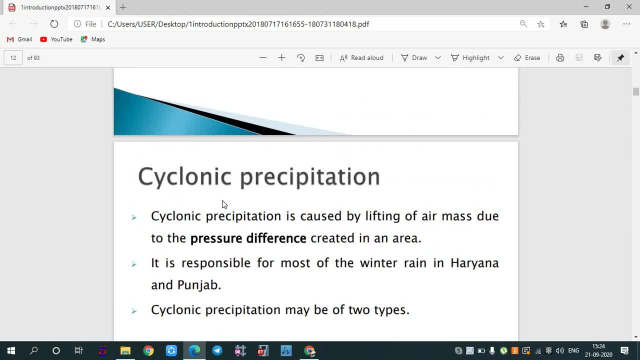 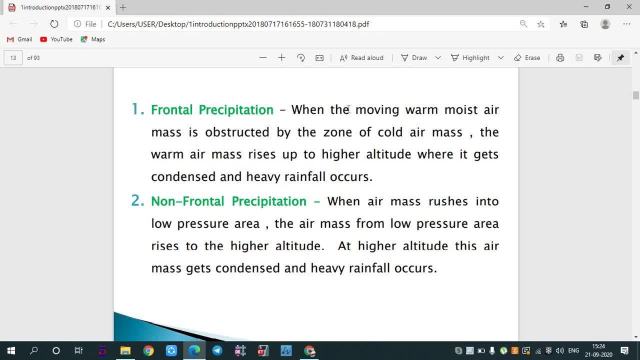 area. now the two category of your cyclonic precipitation is your frontal precipitation, then your non-frontal precipitation. what is your frontal precipitation when the moving warm air? what happened when a moving warm hair air mass is obstructed by a zone of cold air mass? so some moving air mass? uh, warm air air mass is obstructed by a zone of cold air mass. so what? 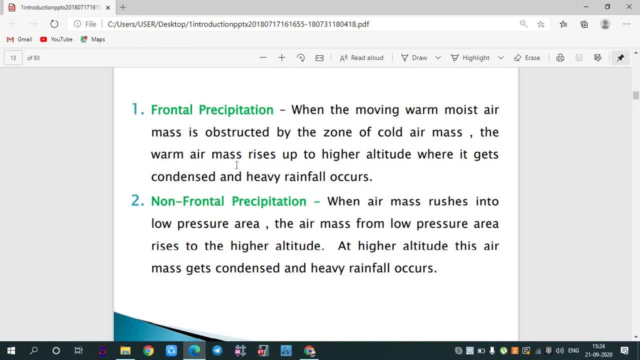 will happen and the warm air will rise up. since it is lighter in weight, warm air generally have less density as compared to cold air, so it will rise up into an altitude where it gets condensed. as it rises, it gets condensed and heavy rainfall occur. so this is your frontal precipitation. what 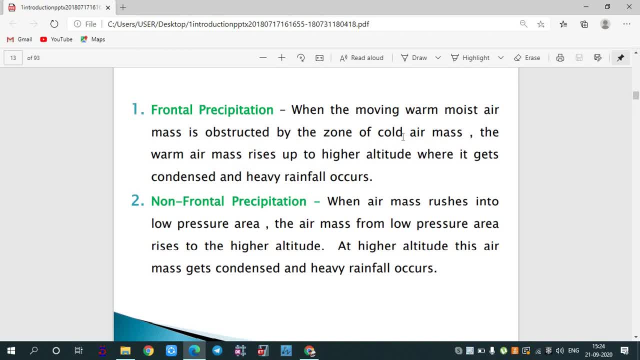 is happening. moving air gets obstructed by cold air mass and because warm air has less density, they rises up. and because it rises up, they condense over there and heavy rainfall, then your non-frontal precipitation when air mass rushes into low pressure area. so when the air mass, what? 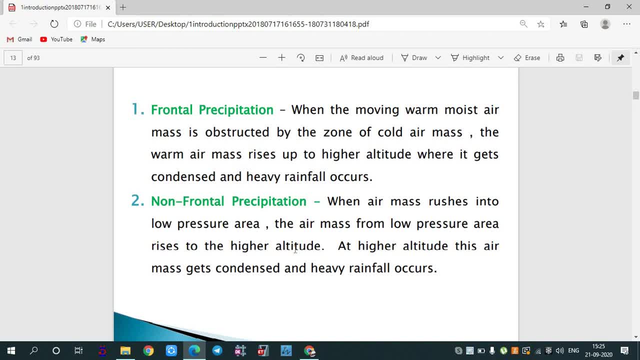 it. when it rushes into low pressure area, the air mass from low pressure area rises to high altitude. so because of the low pressure zone, so this air mass will rise up at higher altitude and over there it will get condensed and again heavy rainfall occur. so this is the 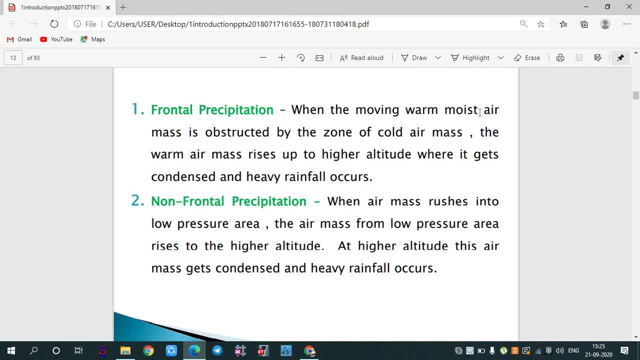 non-frontal precipitation. in this there will be a connection between warm air and cold air. in there, in this world, what is happening? air mass is what rushing into a low area, low pressure area, where the pressure is very low. so in this case also, what happened? the air mass rises. here we just. 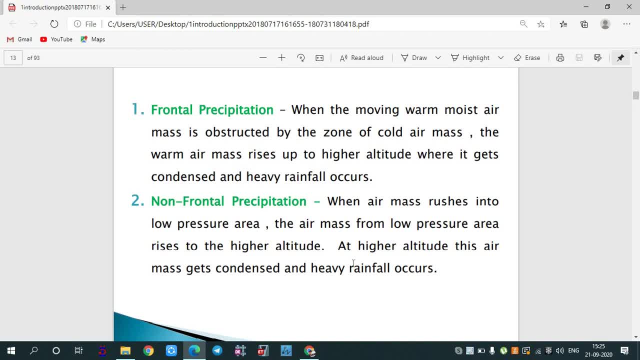 up to higher altitude. and what happens at higher altitude? this will get: the air will rises up, the air will rise up and ultimately it will get condensed over there and what will happen? heavy rainfall will occur. ok, so this is the two form of your cyclonic precipitation. 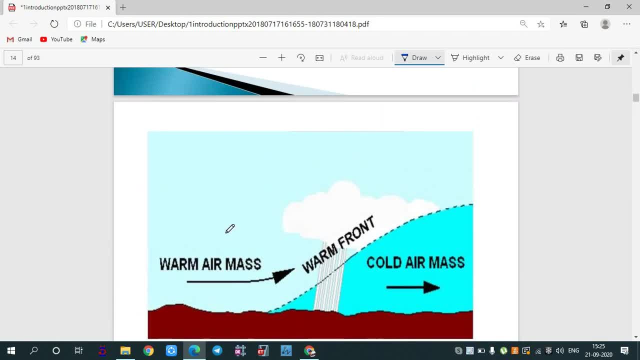 frontal precipitation and non frontal precipitation. as you can see over here, there is a diagram, the warm air mass, and there is a cold air mass. what is happening? this warm air mass get obstructed by what the cold air mass? and ultimately because it is having less density. 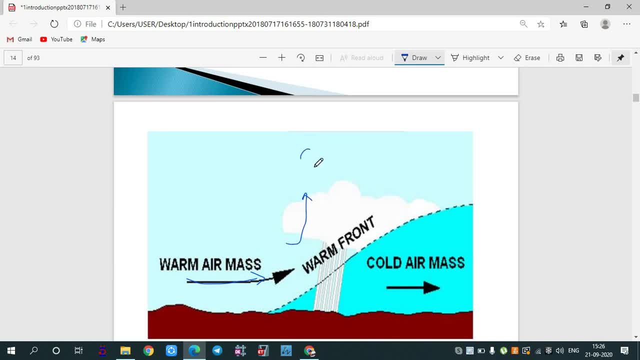 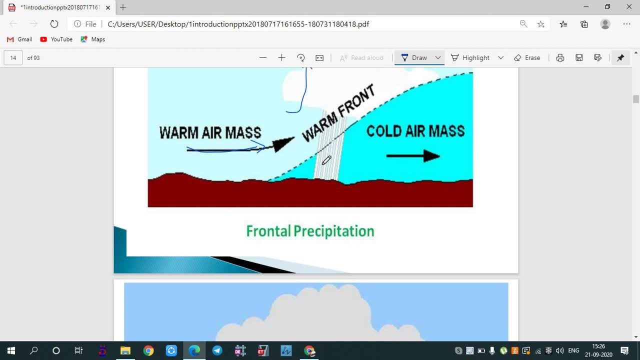 it will rise up and it will condense over here. it will form cloud. ok, and after the formation of cloud, what happens? the precipitation happens in the form of rain, snow sleet. it can be in any form depending upon the region. after that non frontal precipitation, what is happening? 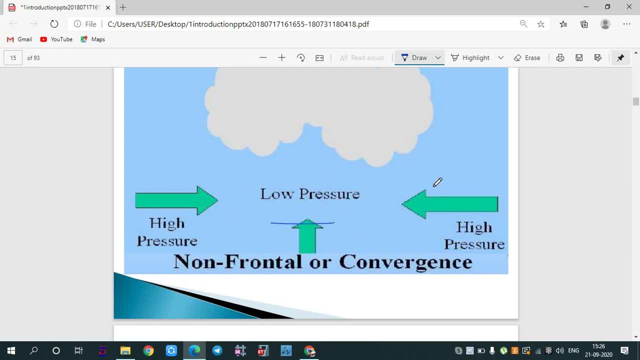 this is the low pressure region. ok, this is the high pressure region. the air mass come. ok, since, because this is low pressure region, the air mass it is travelling over here, it receives at the low pressure region and ultimately it rises up to the higher altitude. over there it get condensed and ultimately 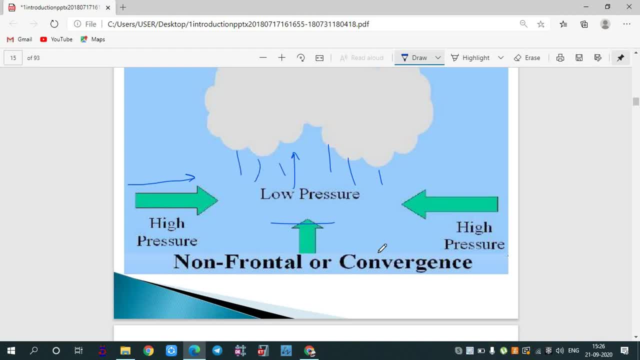 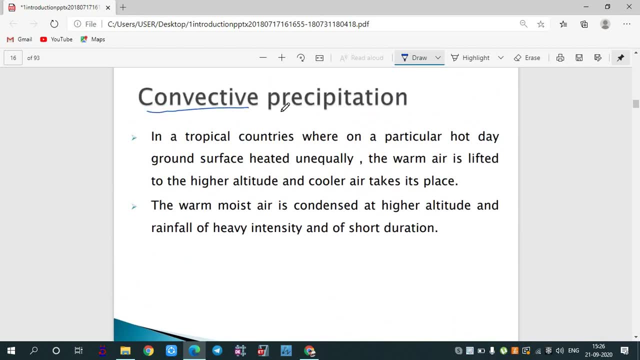 it forms rain. ok, that is your non frontal, or it is also called as coverages. after that we will see the second form, that is your convective precipitation. ok, so And so, basically, it happens in tropical countries. so this represents exactly the same in tropical countries that are not hot in the day and on the day its lower, the temperature is challenge. 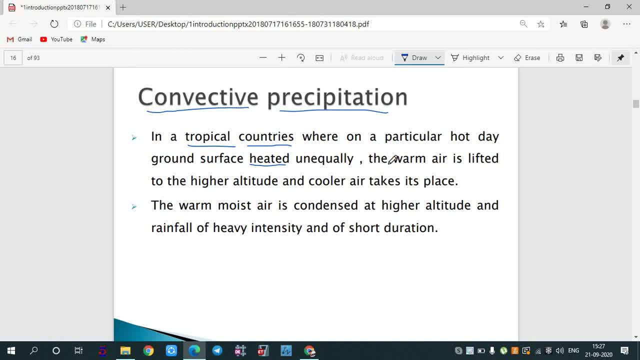 ok. When there is temperature hotter, then the dome is horizontal and it will appear above in mes aspire above and very high temperature. also, it becomes purer and the surface will destroy. so OK, so this happens in only tropical countries where, particularly hot days, ground surface heated unequally ok. and so where on what happens? hot days, ground surface is heated unequally, the warm air mass is lifted to a higher altitude. 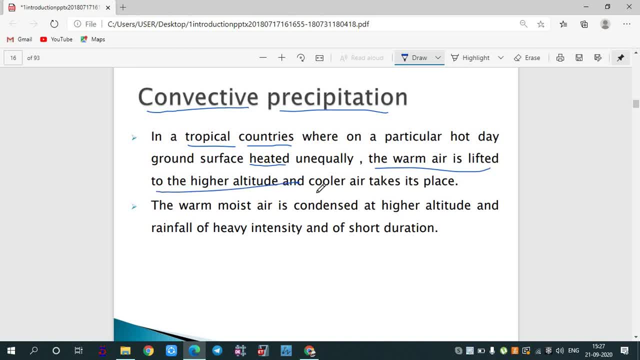 air will get lifted to higher altitude and cooler air take its place, since it is hot during the day. what will happen? the hot air will get lifted up and it has been taken by coolers. cooler air, okay, the warm, moist air is condensed. so this warm air, which is been 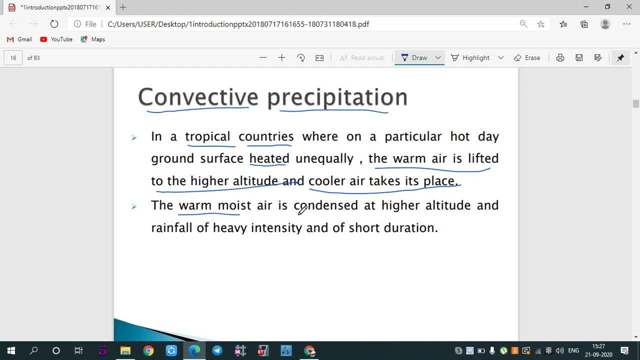 lifted up, will what it will condense over there at higher altitude and it will result into what rainfall of heavy intensity and or short duration. so rainfall can be of heavy intensity also as well as of shortage. so basically, convective precipitation happens in tropical countries where the day temperature is high. okay, so because of the day temperature, 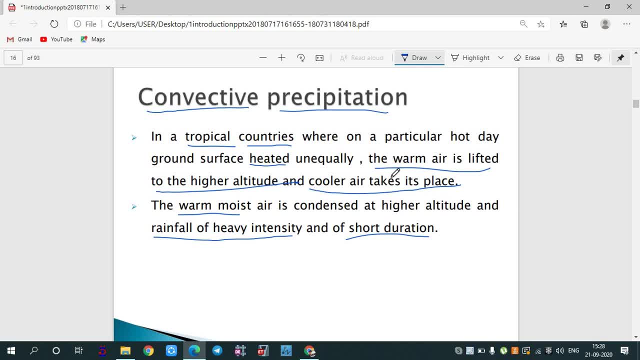 is high, the warm air gets lifted up to higher altitude and the warm air place has been taken by cooler air. the warm, moist air is then condensed at higher altitude and heavy rainfall can occur, as well as, or as well as also some short duration of rainfall, when also happen. 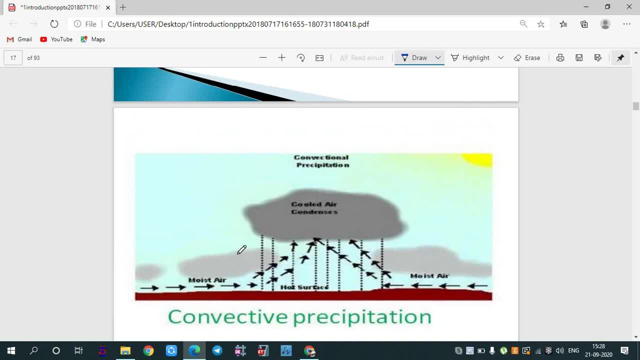 okay, so this is the diagram of convective precipitation, as you can see that the moist air is moving. since this is a very hot surface of the ground, because of this, the moist air get, rises up, it condense over here and it ultimately result into formation of formation of cloud and then 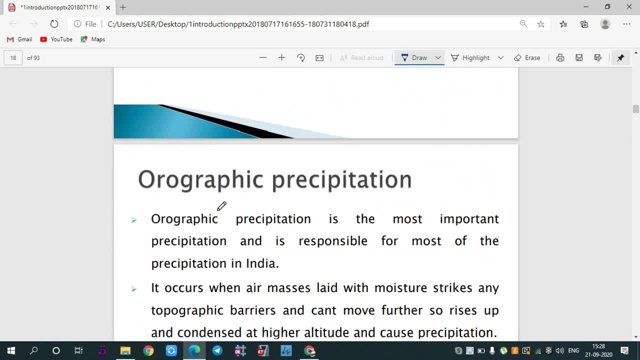 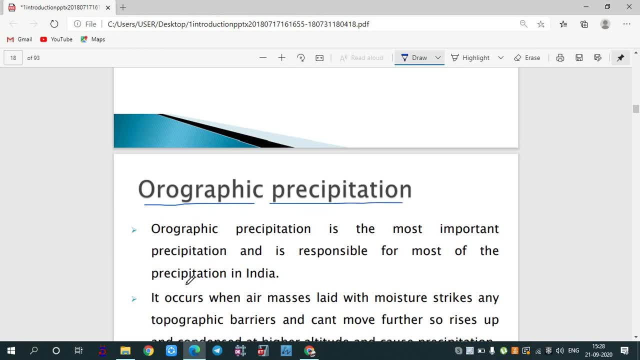 ultimately, what happens? the rainfall occurs. the most common form of precipitation is your orographic precipitation. okay, so this is the main precipitation. okay, so this is the main precipitation. in India, orographucp precipitation is the most important precipitation and is responsible for most the precipitation in india. so, in India, which type of precipitation? 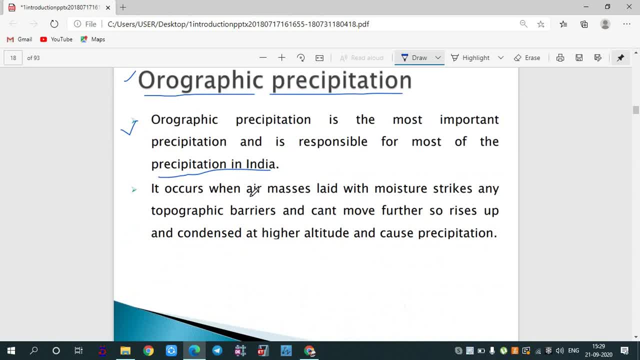 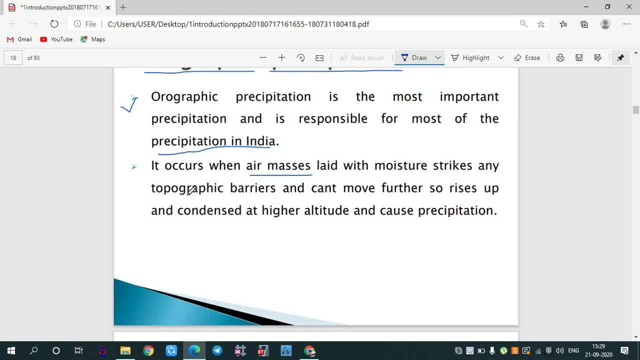 happen? orographucpccp precipitation happens what happens in orographucp precipitation air, which occurs when air mass with moisture strike any tropical tropical barriers and cannot move further, so rises up and condense at higher altitude and cause of precipitation. so what happells? 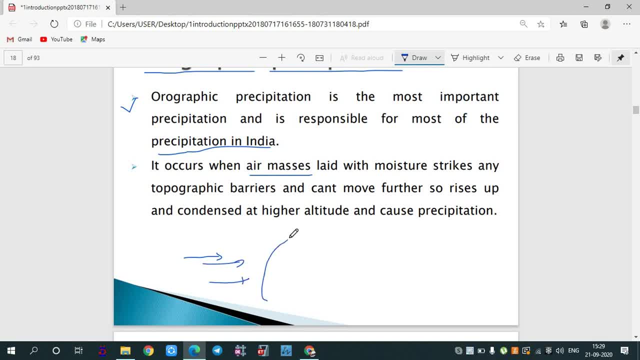 moving. okay, suppose there is a hill over here. what will happen? it can't move further. what will happen? this air mass will now rise up, this air mal. what will happen? this air mass will rise up and ultimately at higher altitude. what will happen? it will condense over there and ultimately result. 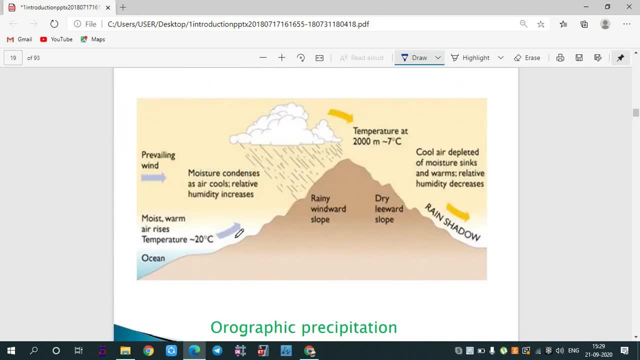 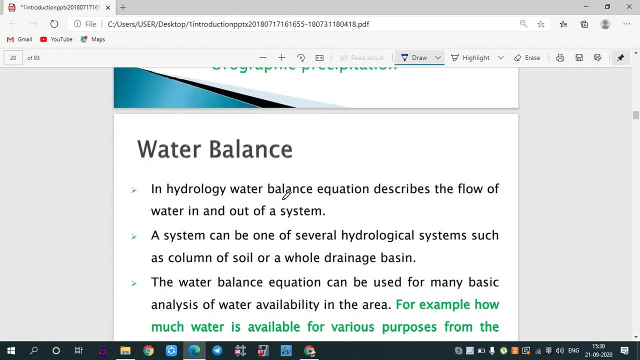 into precipitation. so this is your orographic precipitation. here you can see the diagram. some warm air, moist, is moving over here. since there is a hill over here, it will get what, condensed at higher altitude, ultimately result into rainfall. okay, after that we will see what water balance okay, uh, now in hydrology. in hydrology, water balance equation describe the 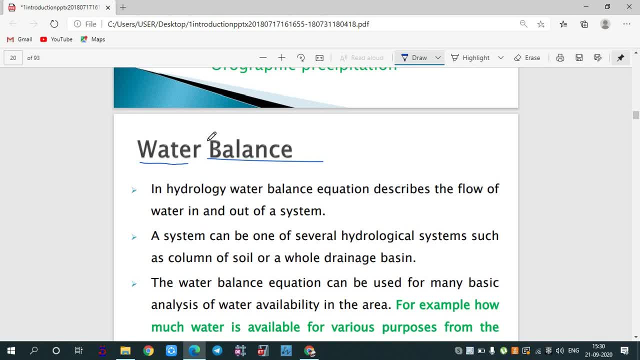 flow of water in and out the system. so, since it is talking about balance, okay, whatever things in hydrological happens, cycle what happens? the water gets evaporated, ultimately get backs to the ground in the form of precipitation. so whatever is coming in, it is getting out. so in: 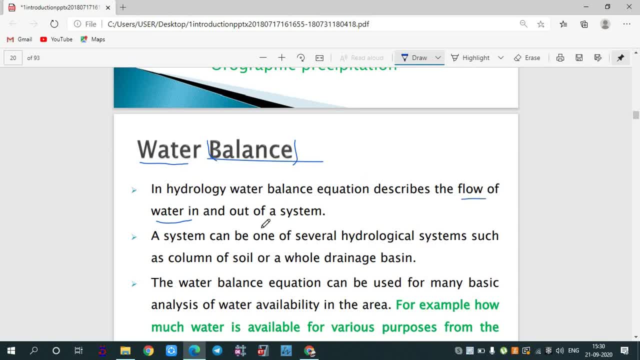 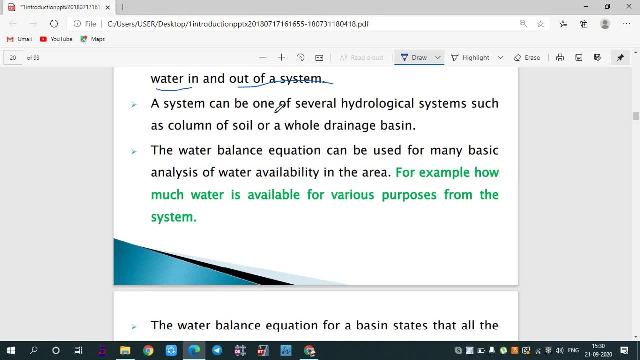 hydrological water balance equation, the flow of water in and out system that we are discussing. okay, now the system can be: uh, now the system can be one of several hydrological system, such as column of soil or a whole system drainage basin. so it is not necessary that we are talking about water balance. 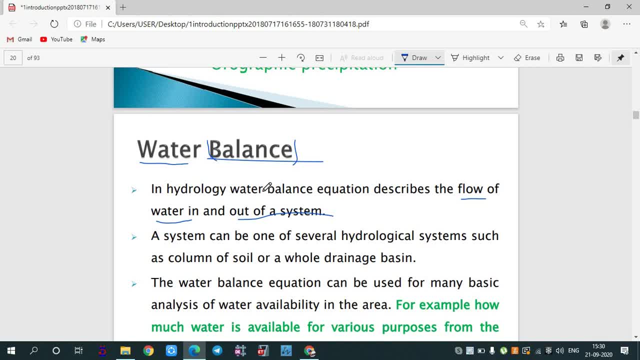 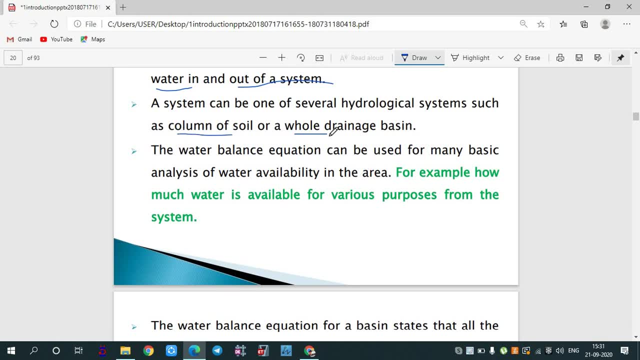 so we are talking about the whole in and whole about hydrological cycle. so it can be a single spring also, it can be a drainage basin also. so it depends on your condition. so if you, if you want to take out for a basin, you will take a basin. consider, you'll consider. 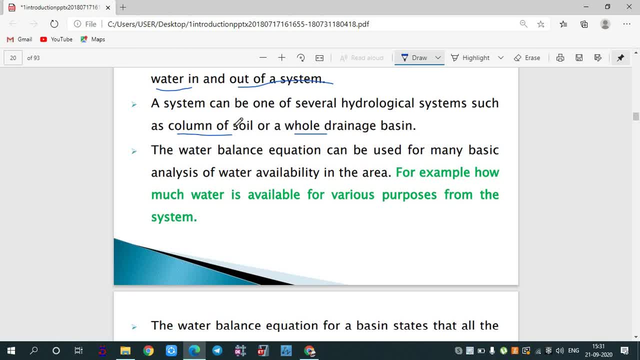 a basin. so if you want the column of a soil, then you will consider the column of a soil. so this equation can be used at various places. okay now, the water balance equation can be used for many basic analysis of water availability in the area. okay, for example, how much water is available for various purposes from the system? 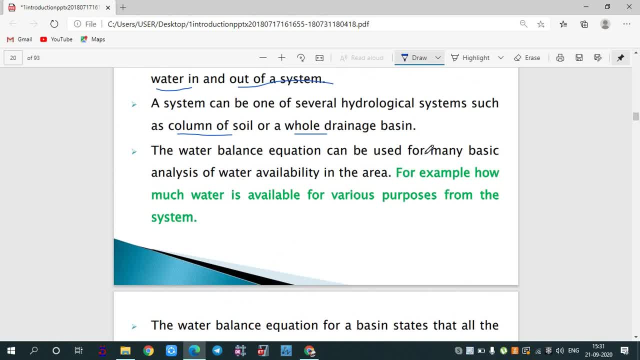 suppose the water balance equation can be used for many basic analysis of water availability in the area. it can be used in various places. for example, how much water is available for various purposes for the system. now, as you can see, the water balance equation for the basin state. 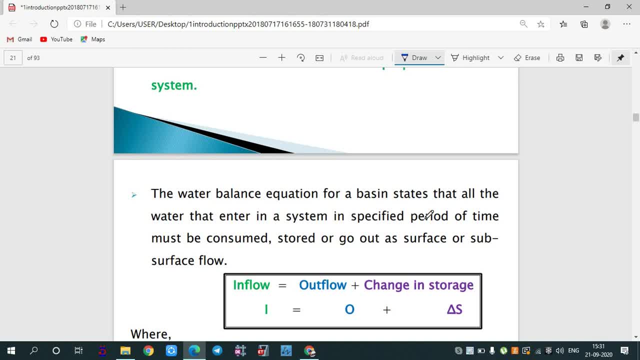 that all the water that enters in the system in a specified period of time must be consumed, stored or go out as a surface or subsurface. so it is saying what, whatever the water is entering in a specific period of time, it must be consumed, or some water must be stored, or it should be go out as a surface or a subsurface flow. so 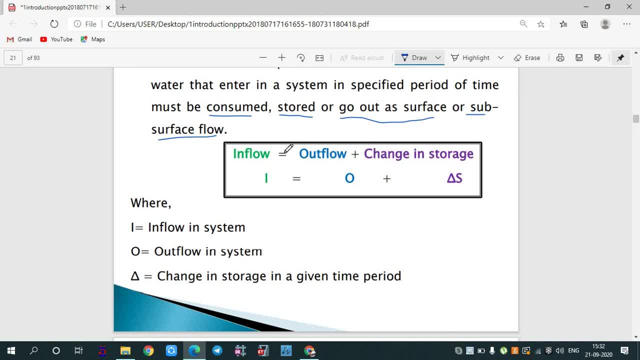 so basically, the water balance. what it is saying: whatever thing is in the flowing, it must be equal to the outflow, or if it is not flowing out, then it must be in the form of a storage. okay, so basically inflow equals to what outflow, or it can be changes. 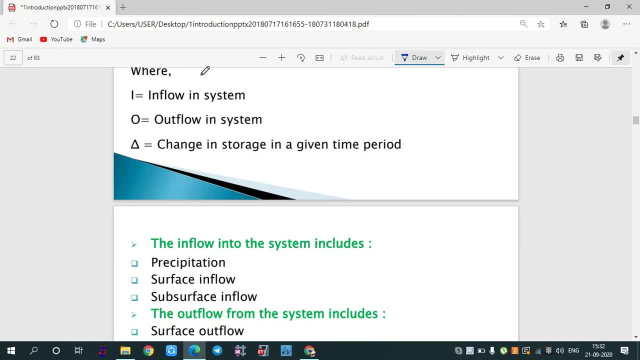 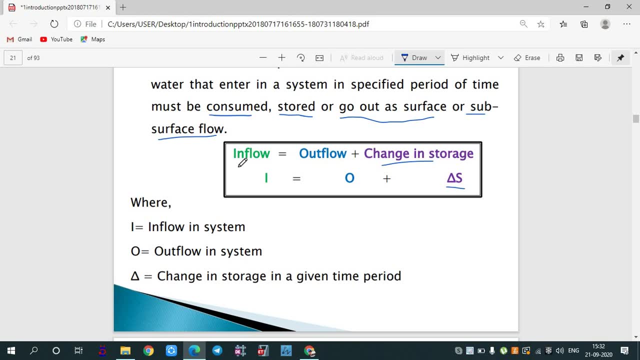 in storage. it can be in the form of storage. okay, so that is your water balance equation. this can be used in various places for measuring what? for finding out different phenomena. so it can be considered for a small drainage basin. it can be considered for a column of a soil. 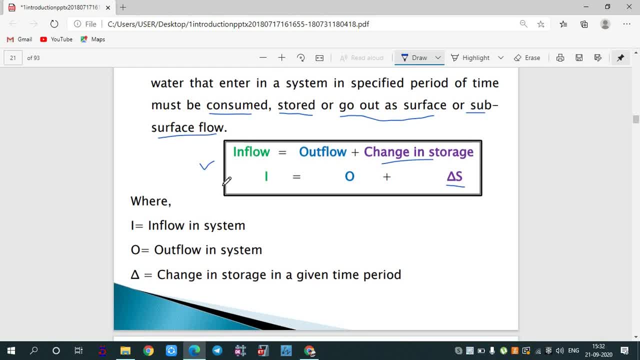 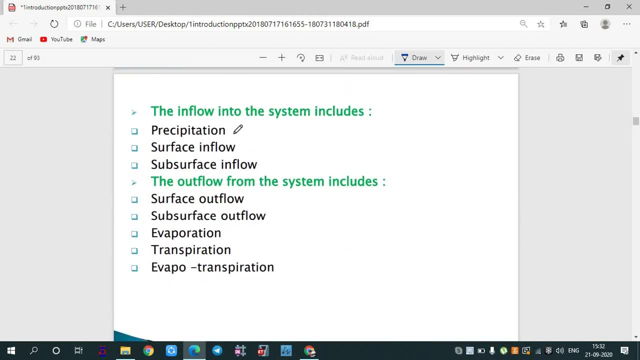 okay, so it depends on your situation. you can use this equation, okay. okay, and now the inflow. if you are talking about inflows a bit, which categories comes under inflow? inflow will be what? precipitation, surface inflow or subsurface. okay, these are the three category of your inflow. now what is the outflow? outflow will be your surface outflow. 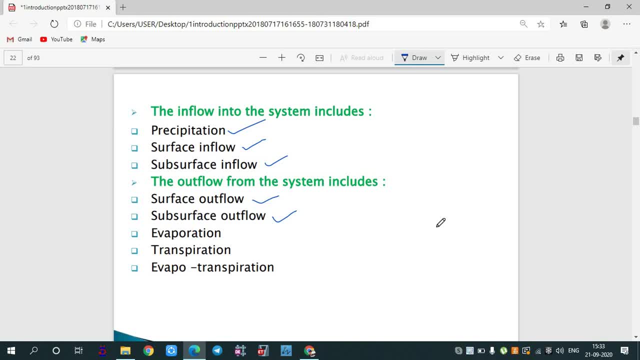 subsurface outflow. as you know, the water will become in the form of precipitation. see again, some water will flow on the surface, that is, in the form of one runoff. some water will flow what inside the ground, that is, your subsurface inflow, now outflow from. 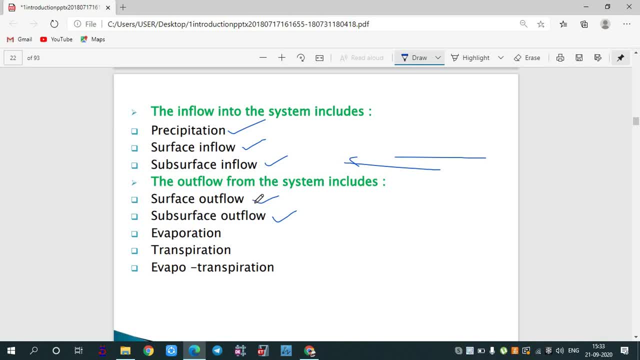 the system now surface out to some. some water will work, some water will get outflow from the surface, some water will outflow from the ground, some water will get evaporate, some water will get transpiration and some water will be evaporate- transpiration. so these are the category of 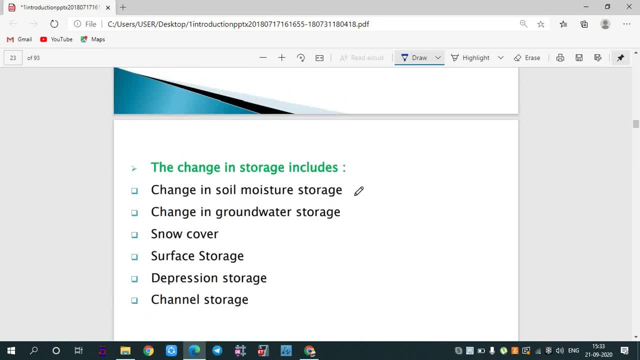 outflow and storage category changes. changes in the storage can be changes in the soil level moisture storage, changes in the groundwater storage. it can be snow covered surface storage, depression storage, channel storage. basically, some water will get stored. it can be in the form of soil moisture storage. it can be. 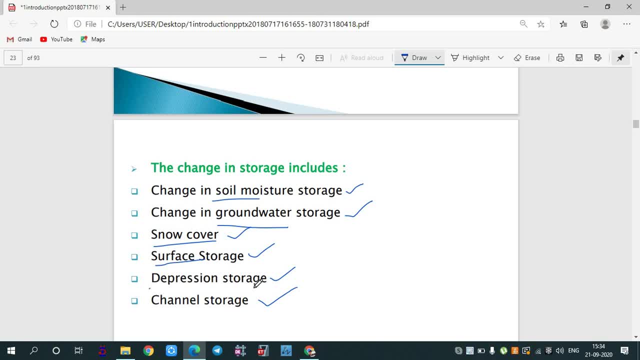 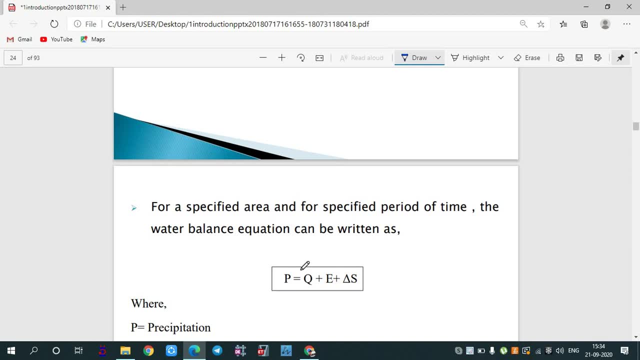 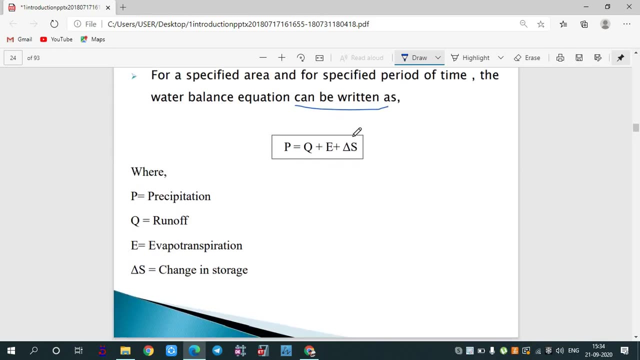 groundwater storage. it can be a snow cover, it can be a surface storage, depression storage, channel storage. okay, now for a specific area, for a specific period of time. the water balance equation can be written as in this form: P equals to odd Q plus A plus del S. so in a brighter form, the water balance.